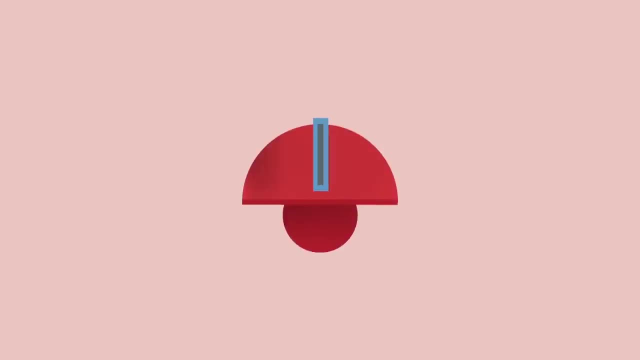 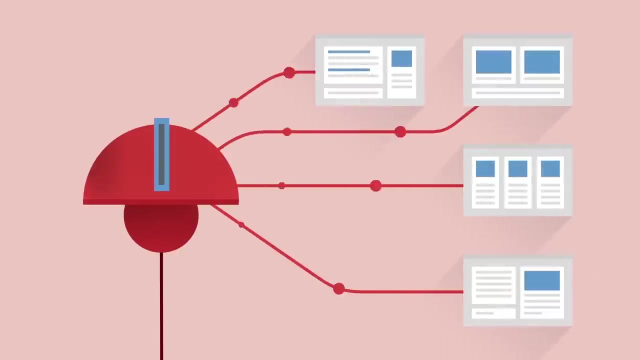 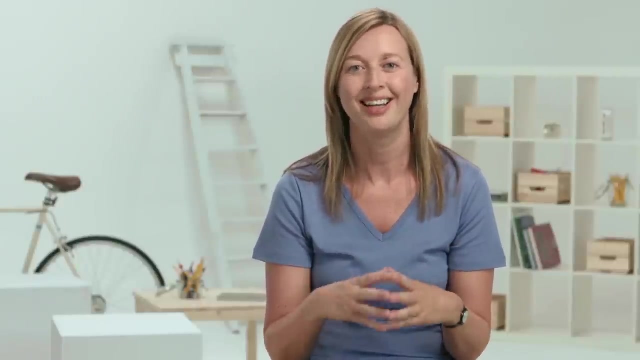 time-consuming. This is where display advertising networks come in. They handle both the buying and the selling of display ads, linking businesses to websites that want to sell advertising space. Another way to think of it is as a marketplace that brings businesses and websites together, helping manage the transactions. There are quite a few of these networks out. 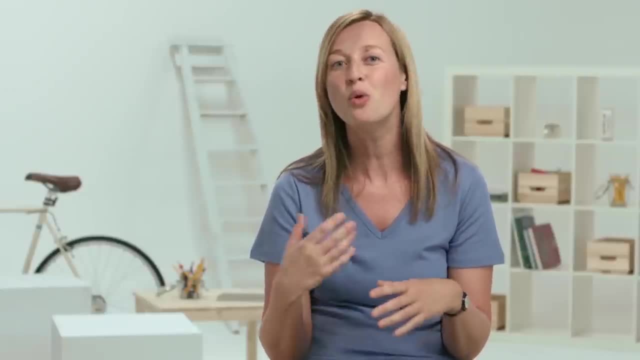 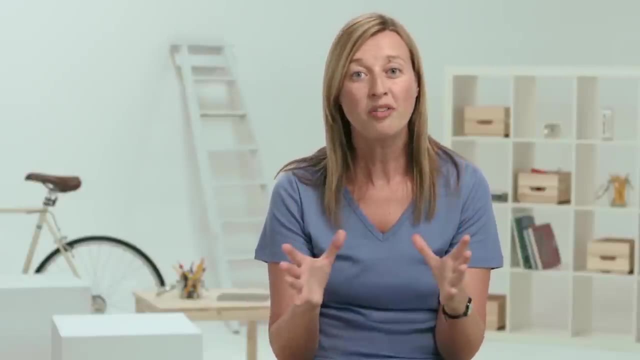 there, like Google Display Network or Yahoo, and they all offer different features, For example, there's a few things most of them have in common. First and foremost, they all offer businesses looking to advertise ad space on the websites, Websites that offer. 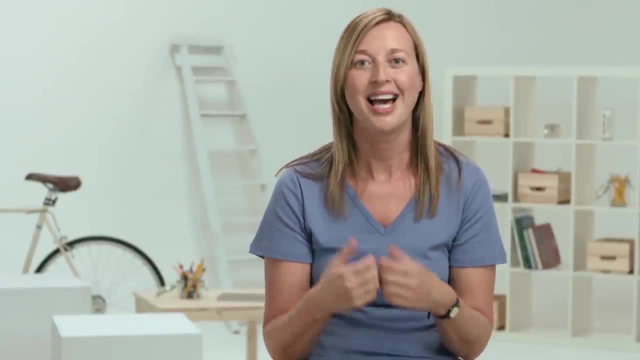 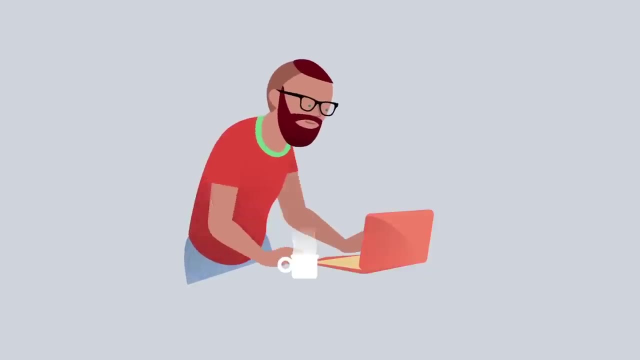 these ad spaces can become part of these networks and they can do things like set minimum prices for how much money they expect for showing ads. Your business can then bid for the spots you want throughout the websites in that network, deciding how much you're willing to pay. 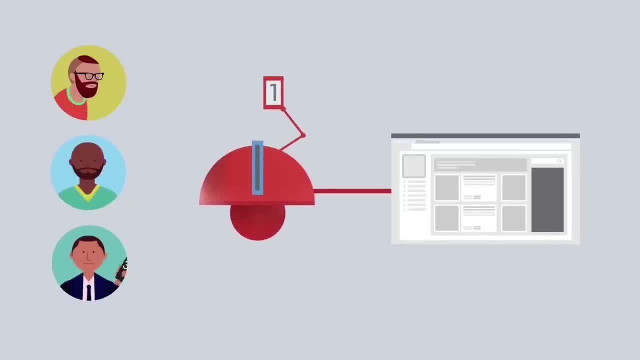 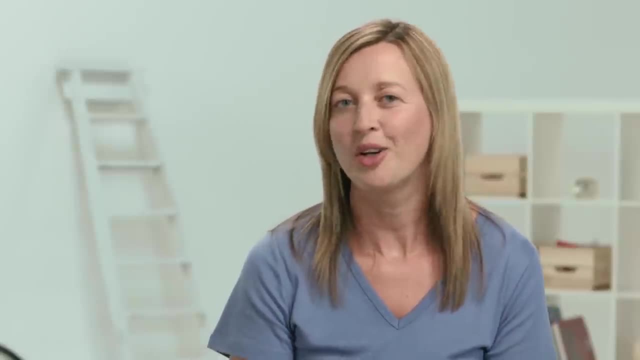 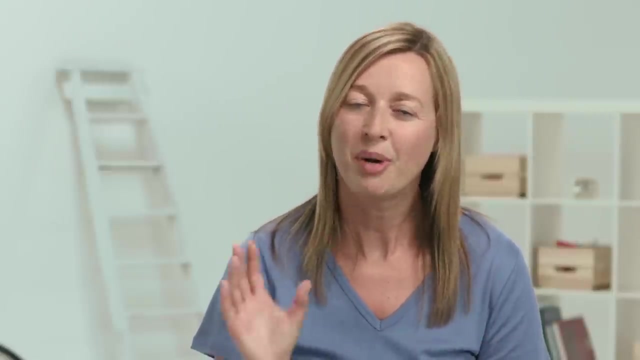 Buyers and sellers are connected. every single time, pages are loaded and the ads that win the right to fill the ad spot are shown. Of course, each network has its own rules, its own features and its own processes and bidding systems, But the key is that they all match. 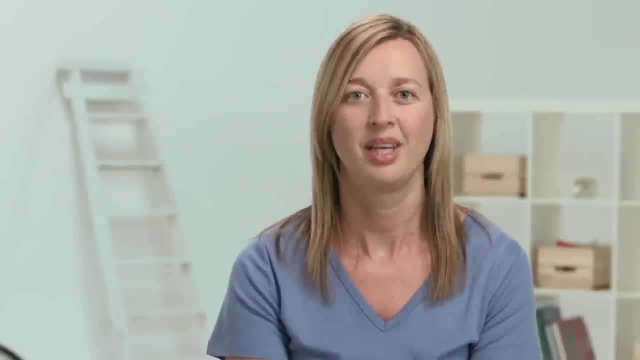 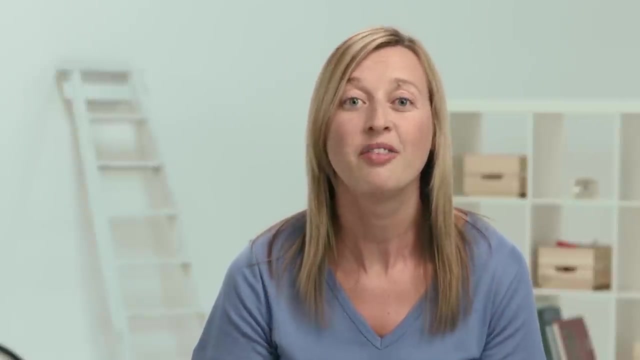 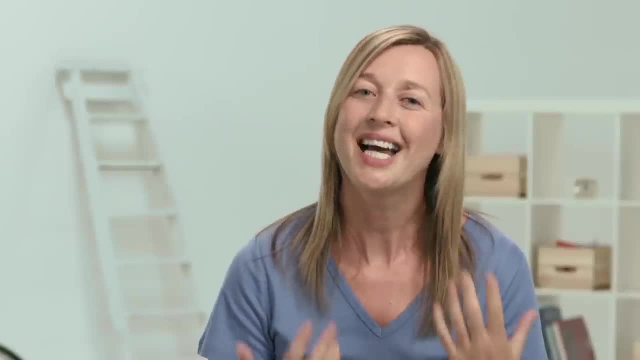 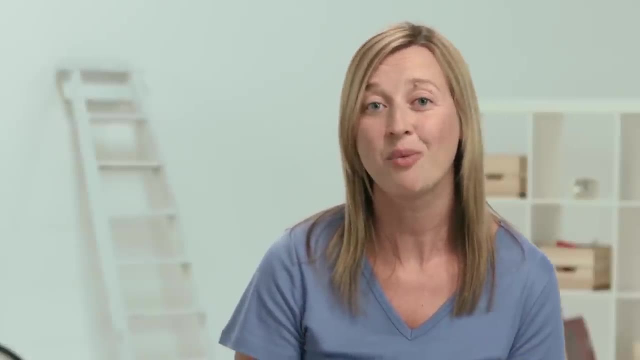 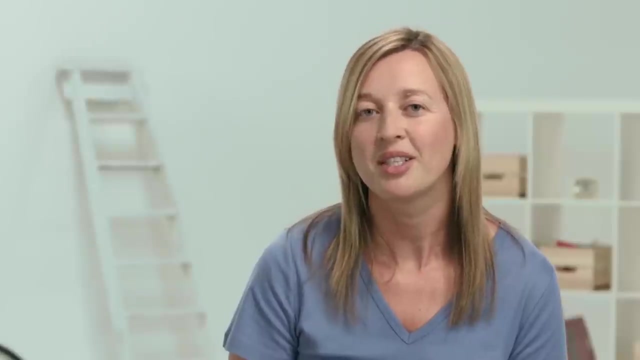 the general information about the people viewing the content. Whilst the exact criteria you can use to find your audience or the way you actually go about running your campaign could vary from network to network, targeting is essential to get your ads in front of the right people. Another thing networks do is handle the money. 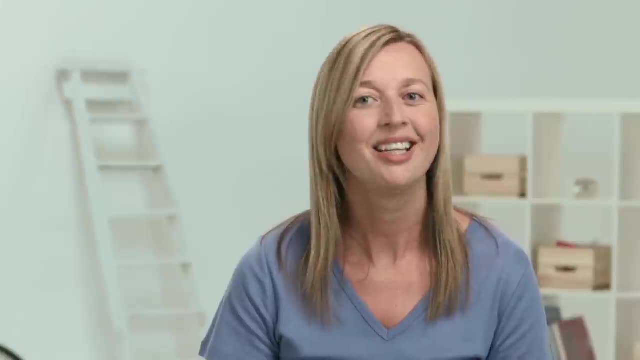 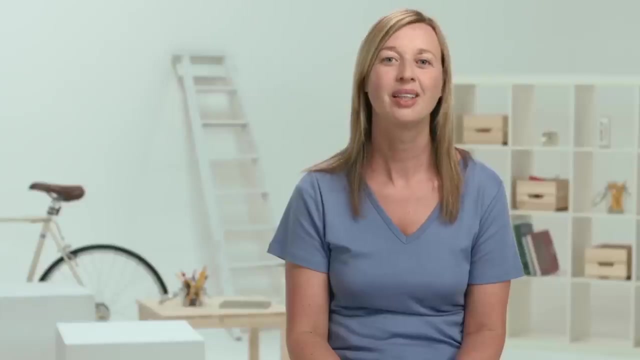 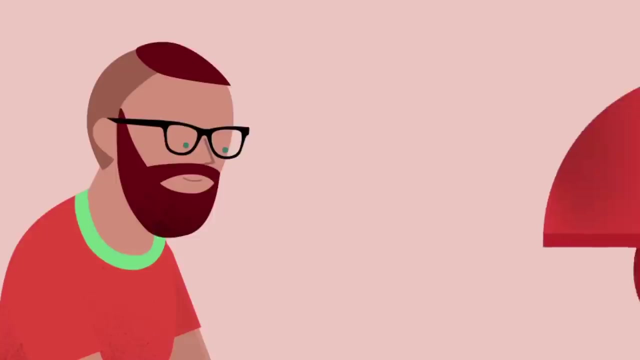 involved. Buying and selling ads happens every second of every day, and the networks collect money from businesses and pay the websites that show the ads. Finally, and perhaps most importantly, advertising networks collect and share data with businesses. They can tell you how many times your ads are shown, how many times they're clicked.